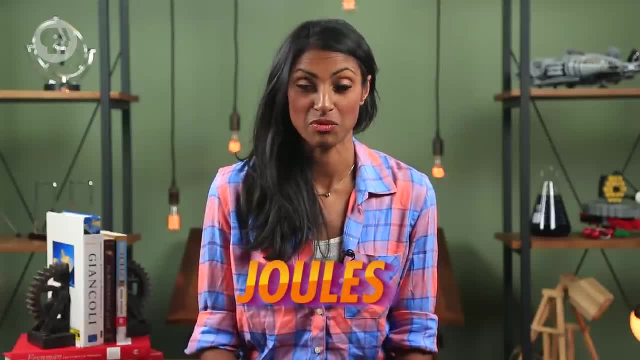 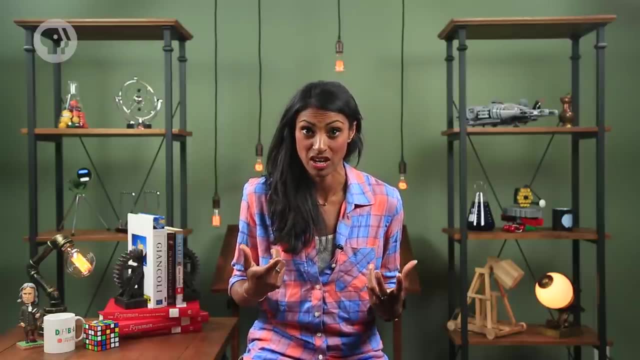 Kilocalories, Or a thousand calories, But in the official international system of units we use joules. One calorie is defined as the amount of energy it takes to increase the temperature of one gram of water by one degree Celsius, or one kelvin. One calorie is equal to 4.186 joules. Simple enough. So the flow of heat changes the temperature of a system, But exactly how much it changes the temperature depends on two things. The first is the system's mass. The more mass a system has, the more heat it takes to change its temperature. 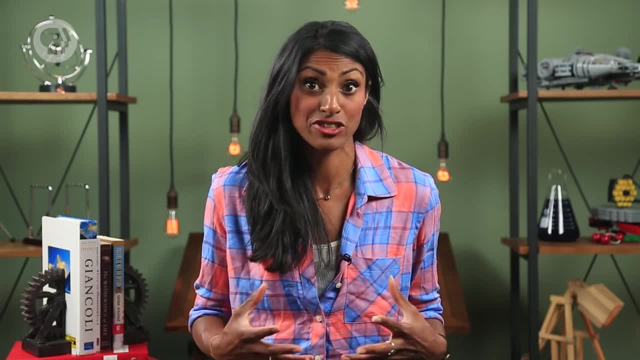 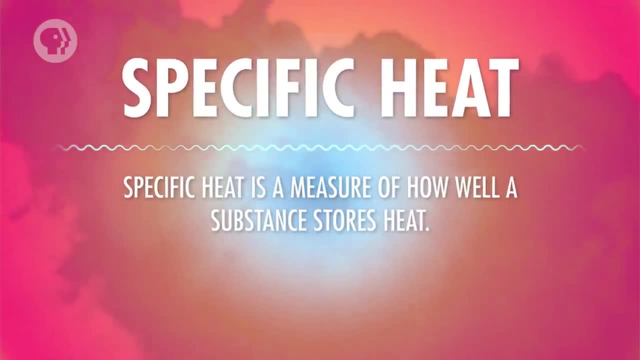 Most systems have more matter after all, so it takes more energy to change its average kinetic energy. But a temperature change also depends on something called the specific heat. Specific heat is a measure of how well a substance stores heat. Every substance has its own specific heat and the higher it is, the more energy transfer. 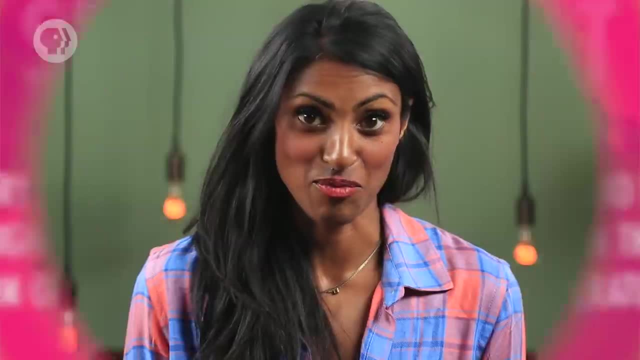 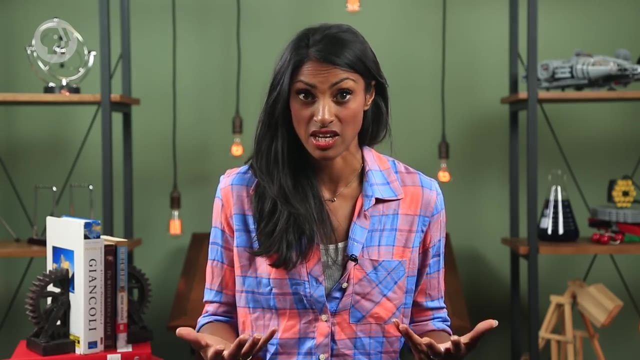 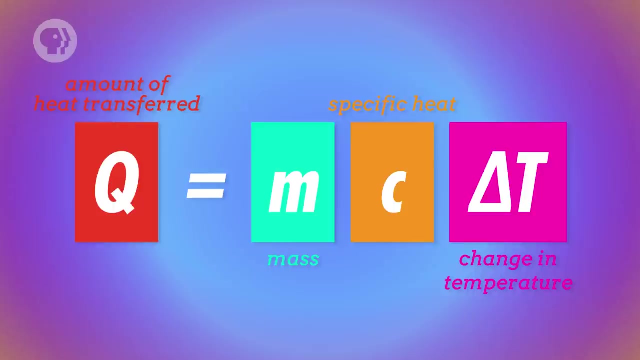 it takes to change its temperature. Water, for example, has a very high specific heat compared to, say, aluminum. That means it takes much more heat to change the temperature of water compared to aluminum. It's equal to the mass times, the specific heat which we designate with a small c. 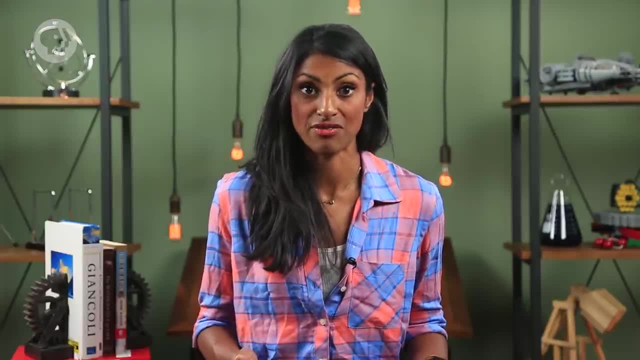 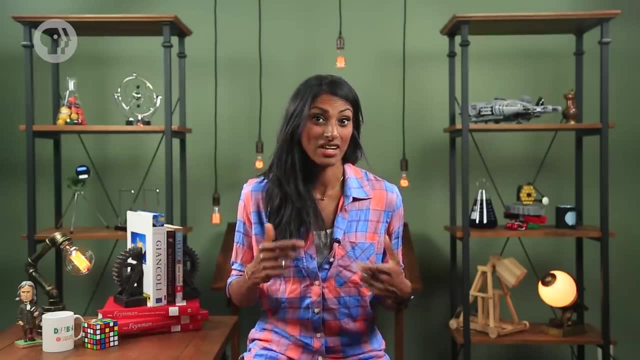 times the change in temperature. And if Q, which represents heat, is positive, that means heat is flowing into the system. If Q is negative, heat is flowing out. But there's another factor that affects the way heat flow relates to temperature. 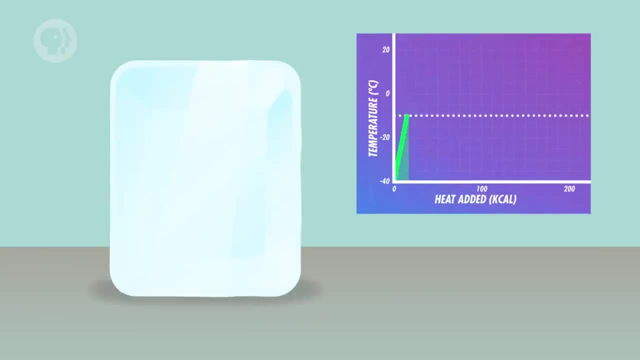 and that is phase changes. Let's say you have a kilogram of ice at negative 10 degrees Celsius and standard atmospheric pressure. Then you start adding heat to it. What happens? Well, we know that the ice's temperature will start to increase. 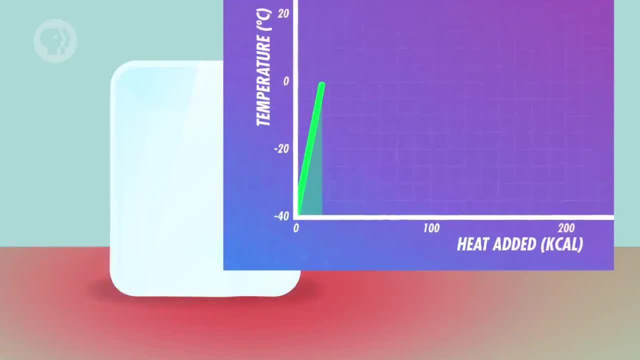 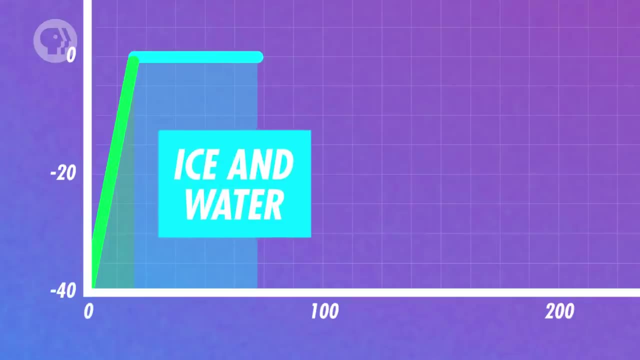 But at a certain point, when the temperature hits zero Celsius, it'll stop increasing because the ice is melting. Then, instead of raising the ice's temperature, the heat you add goes towards changing its phase from solid to liquid, And later, once it's all melted, the temperature of the water increases again as you add more. 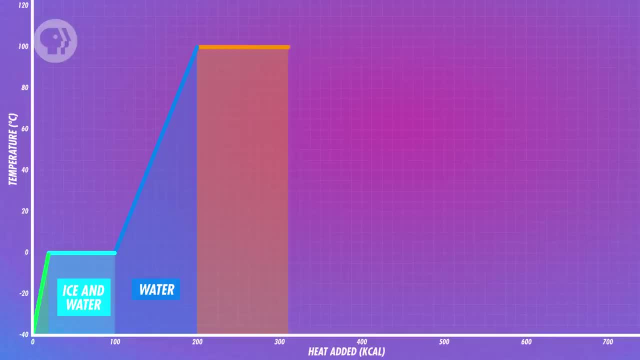 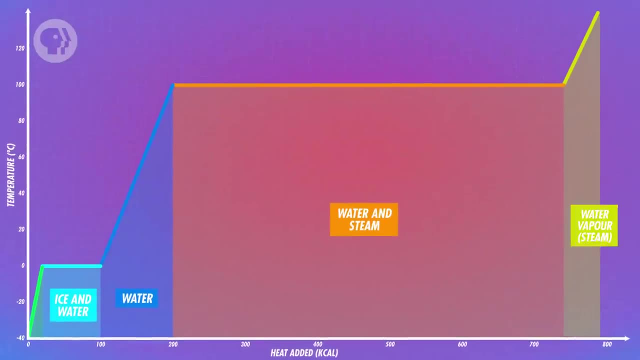 heat until it gets to 100 degrees, And at that point again the temperature stops changing. this time because the water's boiling When all the water has been converted to steam. adding more heat will make the temperature rise once more. So we don't use that earlier equation to describe the heat transfer. while a substance's 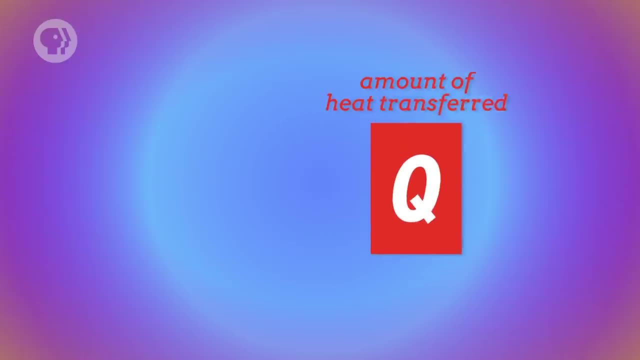 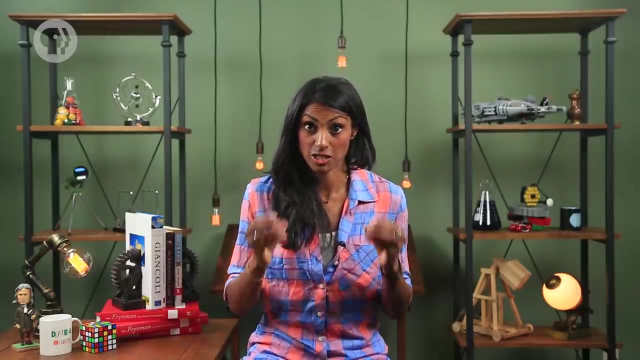 phase is changing. Instead, the amount of heat that gets transferred during a phase change is equal to the mass times, what's known as the latent heat. Latent heat is the heat required to change the phase of a substance And, like specific heat, its value depends on the substance. 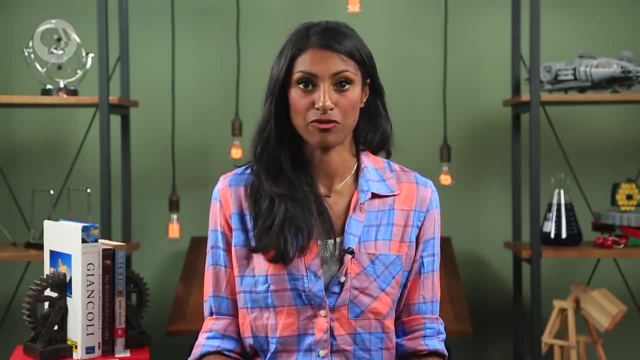 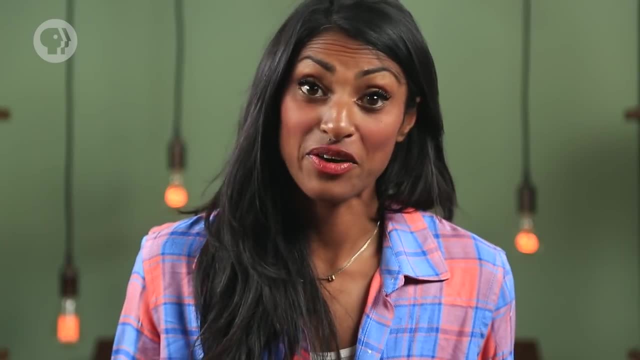 The value also depends on the phase change. For a change from solid to liquid, for example, it's known as the heat of fusion, And for a change from liquid to gas, it's called the heat of vaporization. So that's how heat affects phase changes. 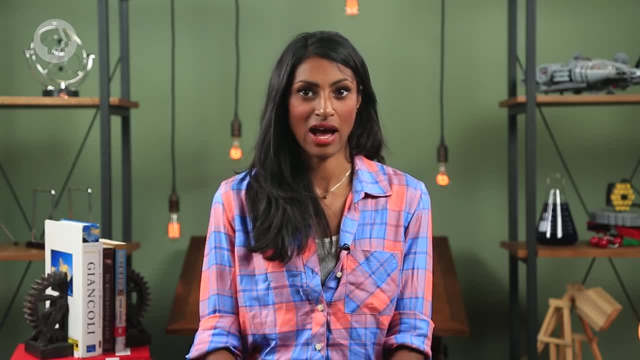 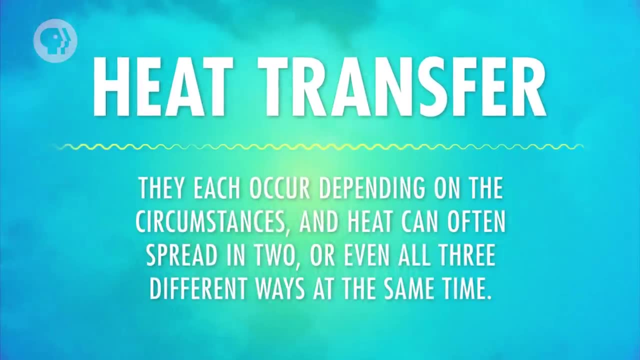 But what about how heat spreads? That's the real key to figuring out why wearing clothes is so great. There are three main ways for heat to spread – conduction, convection and radiation. They each occur depending on the circumstances, and heat can often spread in two or even all. 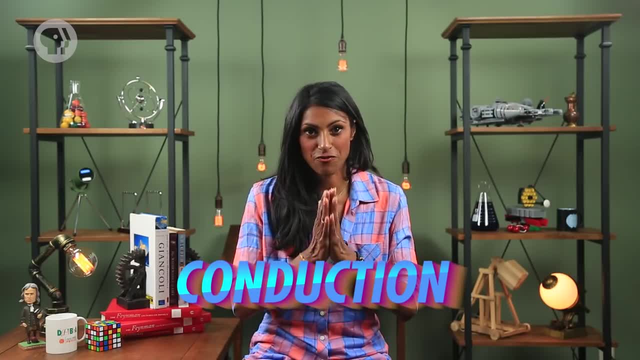 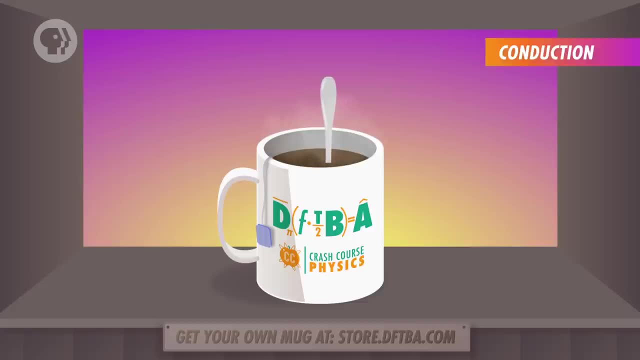 three different ways at the same time. In conduction, heat flow depends on physical contact between molecules which transfer their kinetic energy among each other. It's like when the spoon you use to sew your tea gets warm – heat is conducted from your hot tea to your metal spoon. 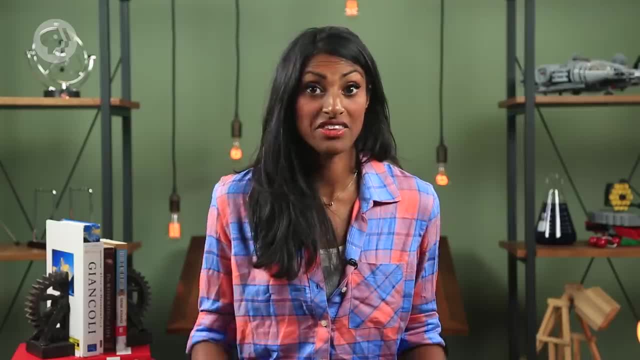 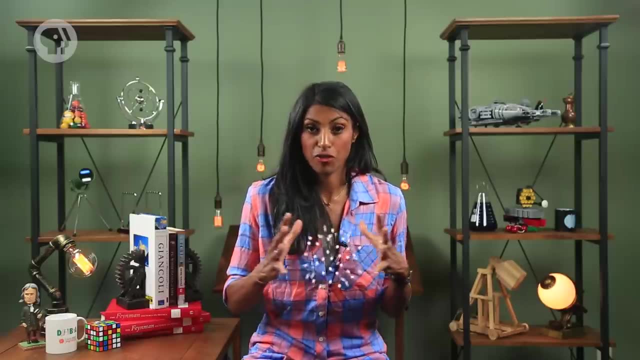 And what determines how much heat will be conducted over time. Well, the bigger the temperature difference between molecules and the bigger the cross-sectional area that the heat's flowing through, the faster the heat flow. But the farther apart the molecules are, the slower it will flow. 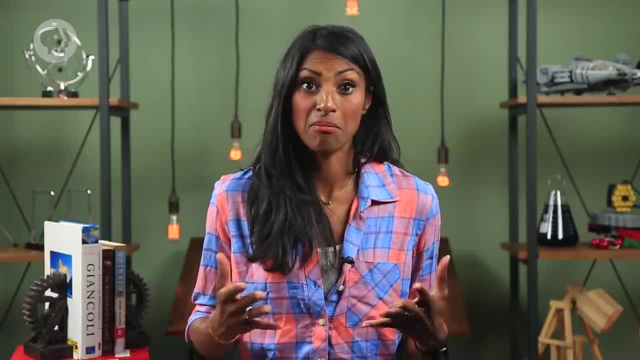 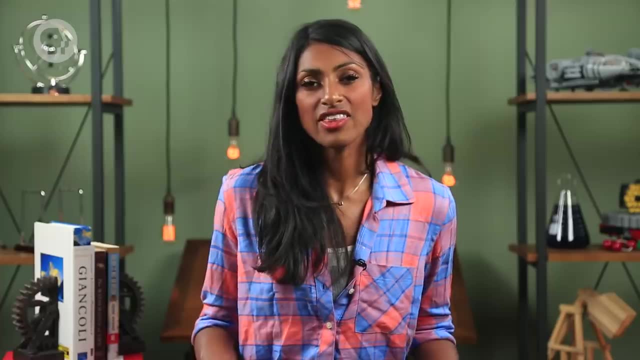 Conductivity also depends on the material. Metal, for example, conducts heat much faster than wood. In equations, we represent this inherent conductivity, known as thermal conductivity, using the letter k. The higher the value for k is, the higher the thermal conductivity of the material. 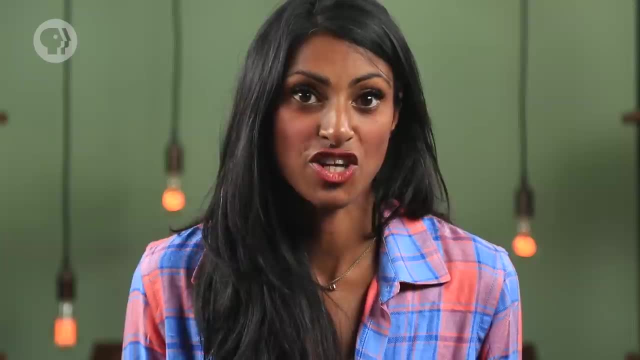 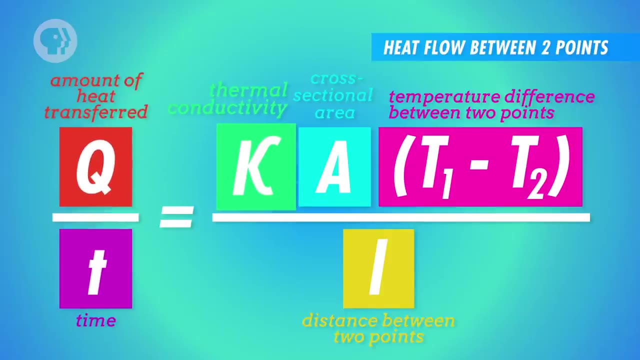 and the faster heat flows. And there's an example. There's an equation for heat conduction over time that puts together all of these different factors. It says that heat flow over time between two points – that's q over t – is equal to. 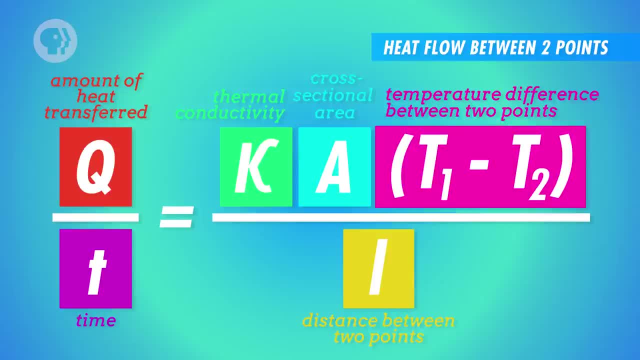 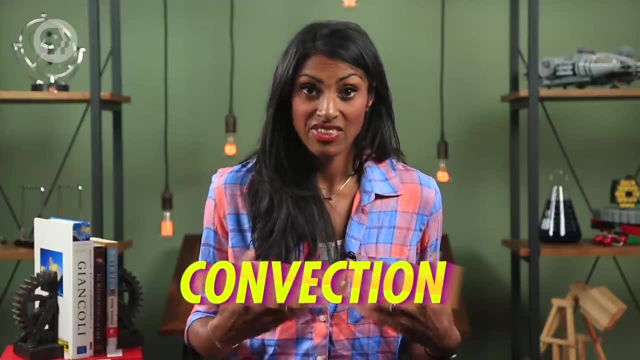 k times the cross-sectional area, times the temperature difference between the two points all divided by the distance between them. Another way that heat can spread is through convection, which is kind of like conduction in the sense that it still depends on contact between molecules. But in convection the molecules aren't just bumping into each other because they happen to be nearby. Instead, they travel much farther. It's kind of like the molecules are being connected to each other. It's kind of like the molecules are being connected to each other. 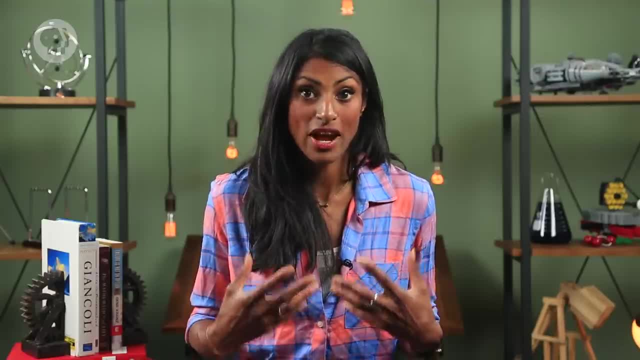 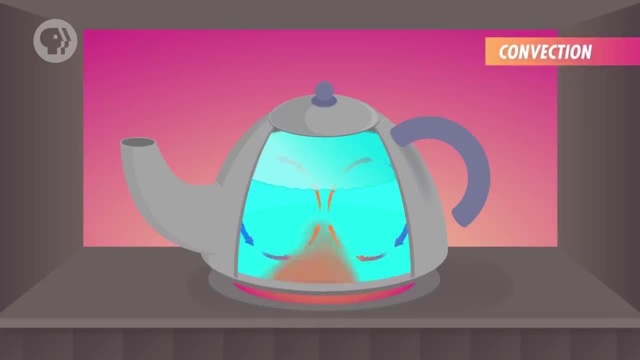 It's kind of like the molecules are being stirred In convection. warmer molecules generally move away from the heat source and are replaced by cooler molecules which are then heated up. In a tea kettle, for example, the water is heated from the bottom, so the water at the 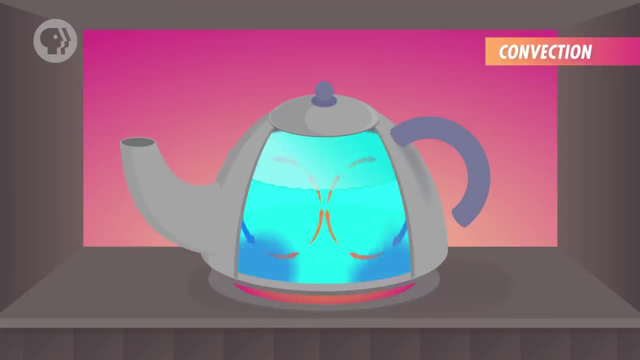 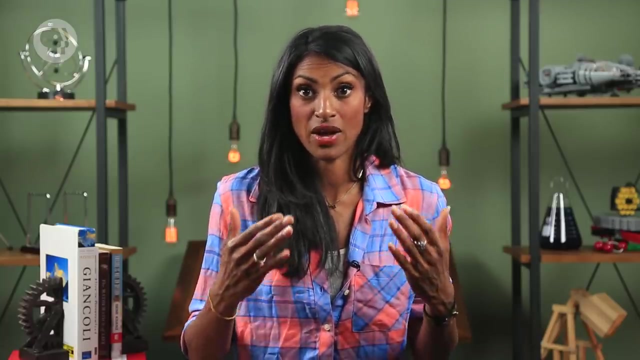 bottom warms up first. That warmer water expands and rises and is replaced by cooler water, which then also heats up. But convection only happens because the heat source is positioned in a way that makes the warmer water move away from it – it's at the bottom of the kettle. 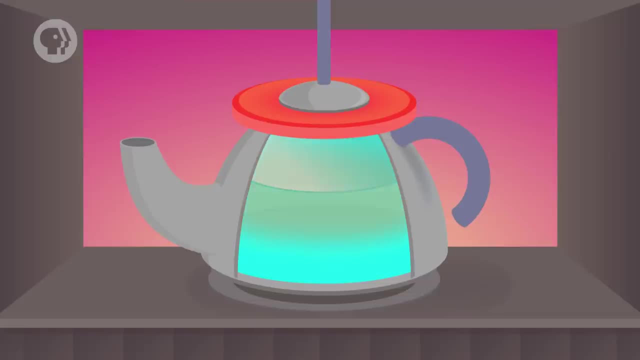 If the heat source were at the top of the kettle, the water at the top of the kettle would warm up first and it would basically stay put, so the colder water wouldn't be able to take its place. As a result, the warm and cold water wouldn't get mixed around, so it wouldn't be heated. 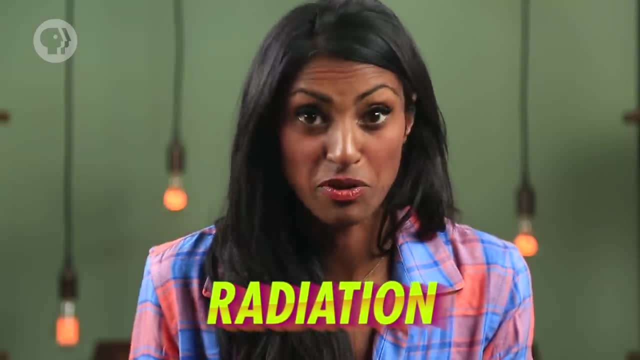 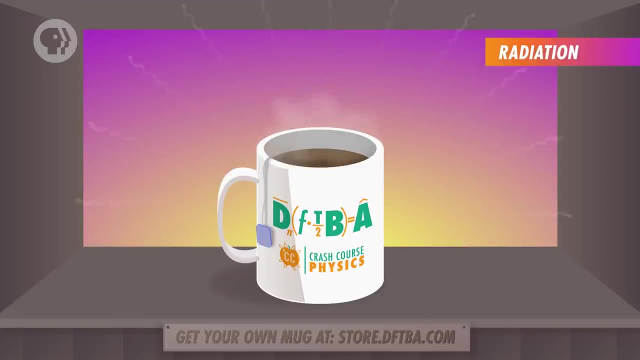 by convection. Finally, there's radiation which doesn't depend on the movement of molecules. Instead, heat is transferred by electromagnetic waves. We normally consider the infrared part of the spectrum to be heat, And we can describe the way heat radiates from an object over time with an equation. 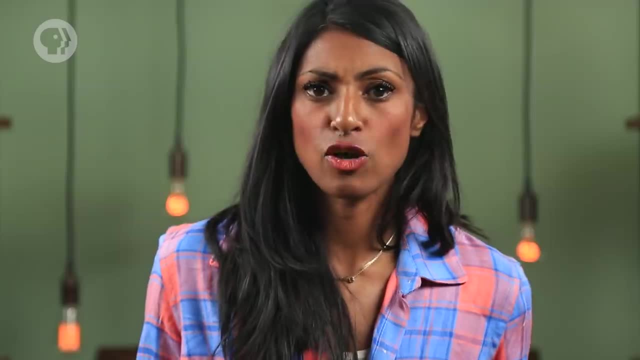 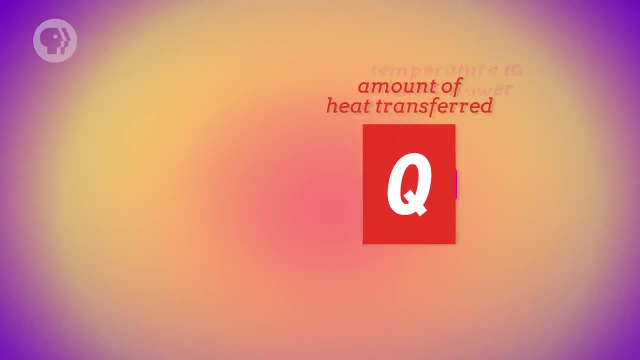 just like we do for conduction, but this one works a little differently. The bigger the object's area, the faster it will radiate, And the same is true for temperature. Specifically, the amount of heat that an object radiates over time is proportional to its 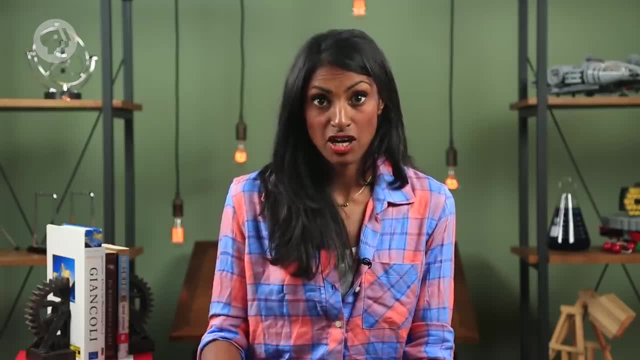 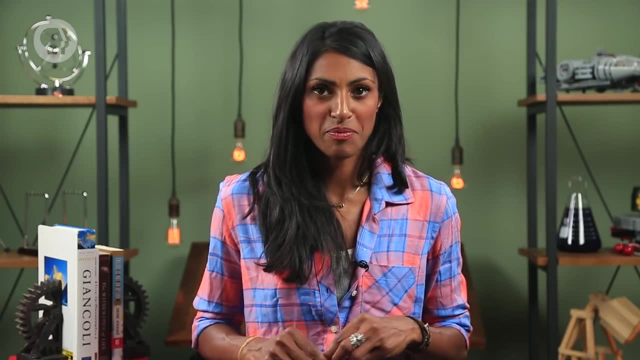 temperature raised to the fourth power Meaning. if you double an object's temperature, you multiply the heat it radiates over time by 16. So temperature's a big deal when it comes to radiation. But radiation also depends on what's known as the emissivity constant, which is based 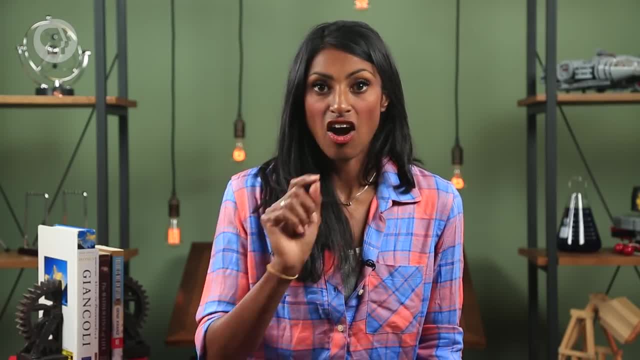 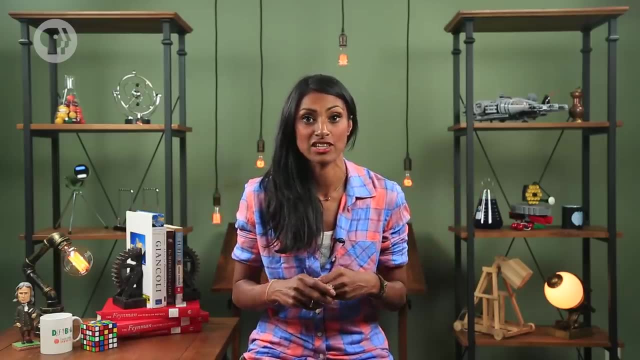 on a material's inherent ability to radiate heat: The higher the emissivity constant, the more it radiates. The equation that combines all these variables together to make up this equation is called the Stefan-Boltzmann equation, to describe how much heat an object radiates over time. 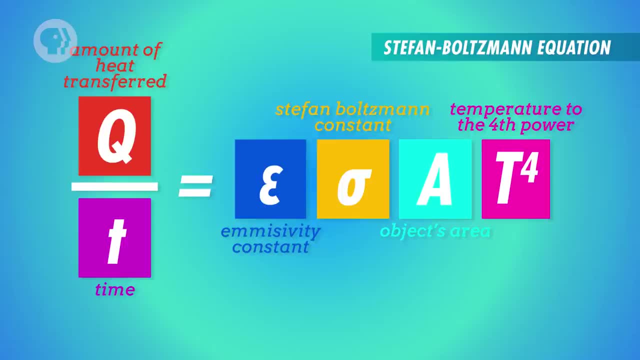 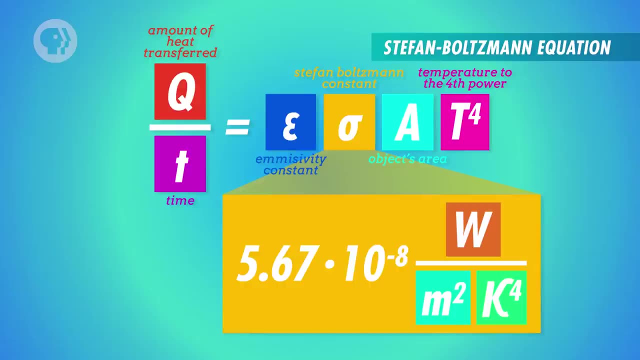 And it says that the heat emitted over time is equal to the emissivity constant times, a special number known as the Stefan-Boltzmann constant times, the object's area times, temperature raised to the fourth power. Now that we've gone through all the different ways that heat transfers, we can finally answer. 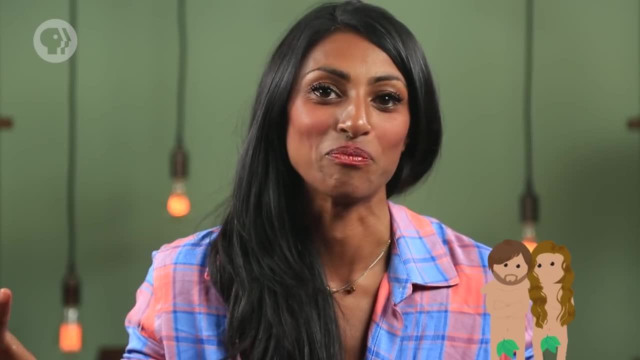 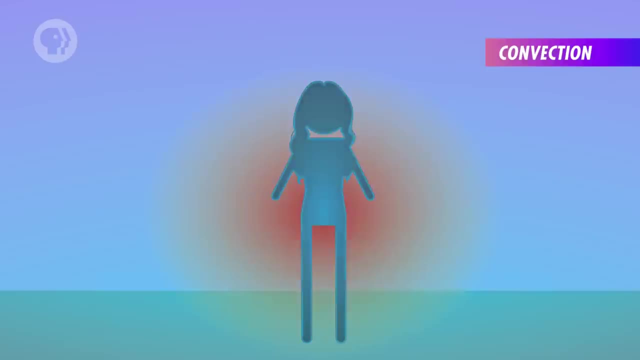 the pressing question: why do we wear clothes? Well, it's simple. Otherwise we'd lose a lot of heat. Your body loses heat in all kinds of ways. One of the main ones is convection. If your skin is warmer than the surrounding air, then you'll transfer heat to the air. And air moves around a lot. so pretty soon the warmer air gets swept away and replaced by cooler air, and you lose more heat from heating up that replacement air. Clothes help by trapping air against your skin. Sure, you lose heat as you warm up that air, but then the warm air stays close to your. 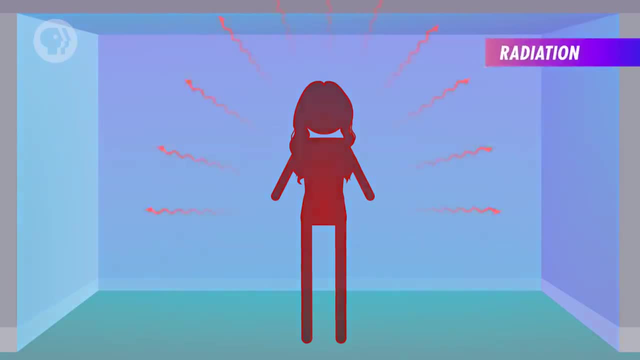 body so you don't lose too much more. You can also lose heat through radiation. If the walls, floor and ceiling of the room you're in are colder than you, you'll radiate more heat to them than they'll radiate to you. 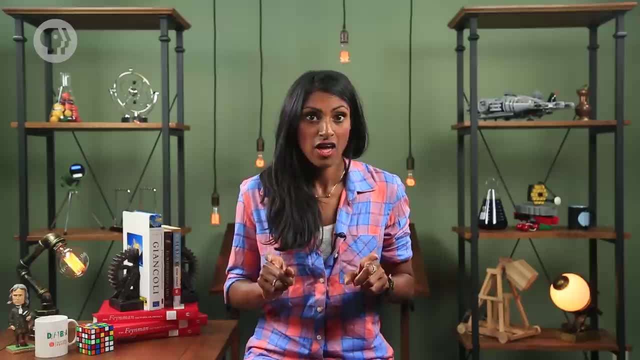 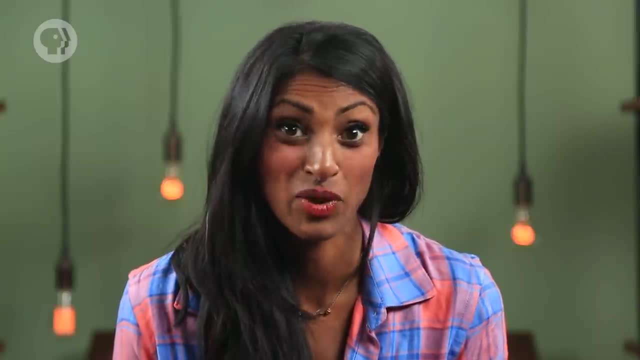 Clothes don't stop you from radiating heat, but they can keep you warm enough for the heat that your body produces to keep up with the heat you're losing through radiation. Just another good reason to stay dressed Whenever possible. Today, you learned about thermal energy as well as heat, and how much of it you need for. 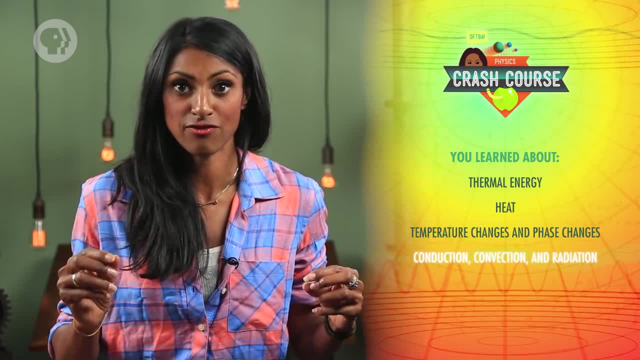 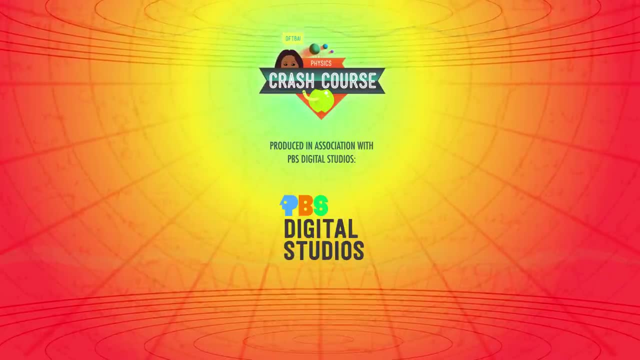 both temperature changes and phase changes. We also talked about heat flow through conduction, convection and radiation. Crash Course Physics is produced in association with PBS Digital Studios. You can head over to their channel and check out a playlist of the latest episodes from.